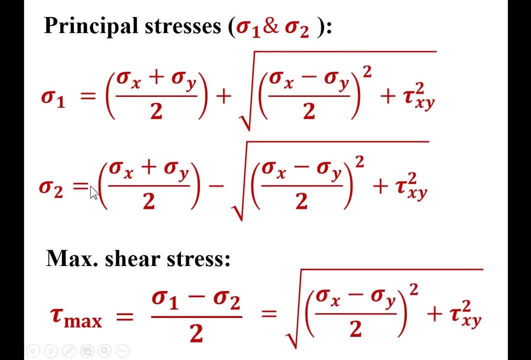 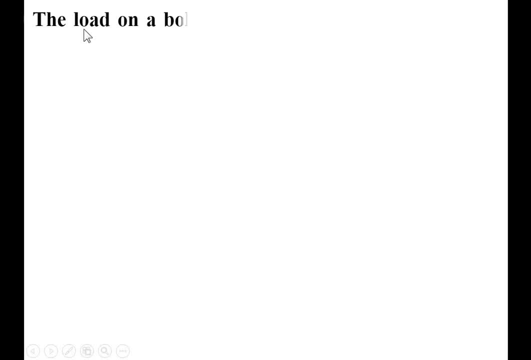 it is the second part of the sigma 1 and sigma 2, so that you have to remember. So now let's start from the description of the problem. So the load on a bolt consists of an axial pull of 25 kilo newton together with a transverse shear force of 10 kilo newton. 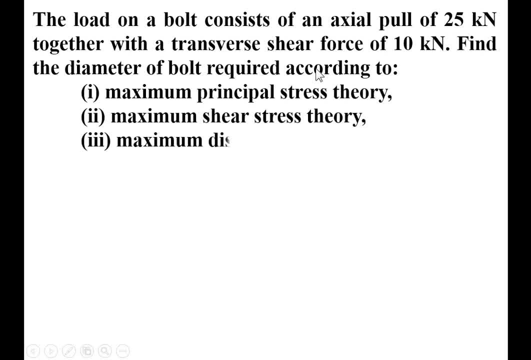 Find the diameter of the bolt required according to maximum principal stress theory, Maximum shear stress theory and maximum distortion energy theory. Take permissible tensile stress at elastic limit as 120 mega pascal. so first of all given data, So that is given to you. the bolt consists of an axial pull. 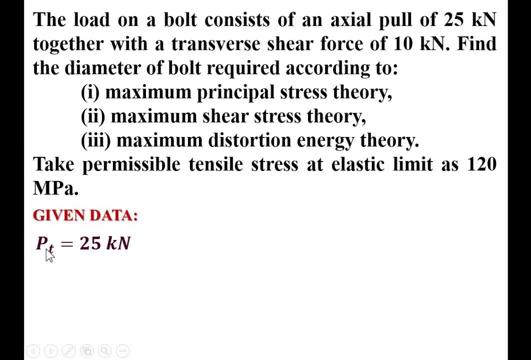 that means the tensile force. so you can say it is tensile force, 25 kilo newton, together with a transverse shear force, so I can say it is a PS shear force, that is, 10 kilo Newton. fine, the diameter of the bolt that. 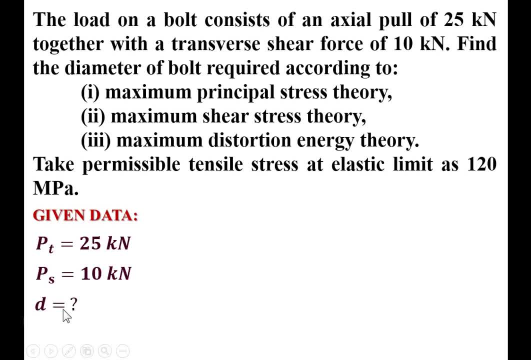 means. D is the question mark. that means diameter of bolt. that is my objective, according to maximum principle stress, according to maximum shear stress and according to maximum distortion energy theory. take permissible tensile stress and elastic limit is 120 megapascal. so this is what we can say s y, T, and you know that mega Pascal, that is what Newton per mm square. so you, 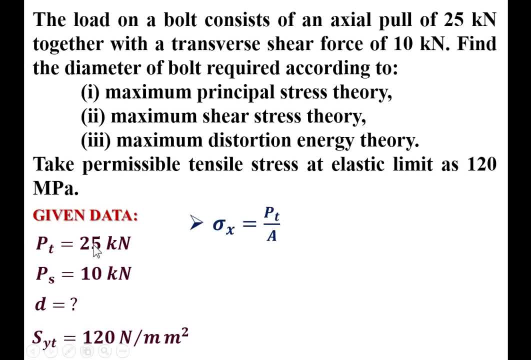 know that stress is equal to load upon area, and here this is axial load. so you can say: the stress produced in the x direction is equal to load upon area, and load is given to you as 25 kilo Newton. so I can put it over here. so PT is 25 kilo Newton. that means 10 raise to 3. 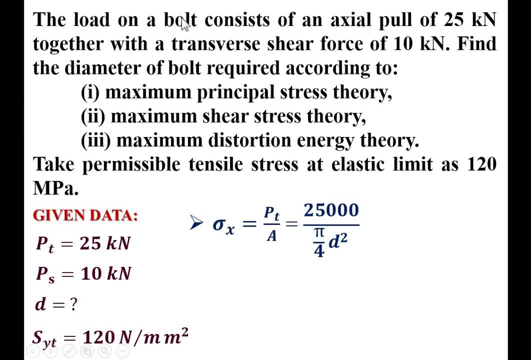 upon area. so you know that the cross-section area of the bolt is circle and so that it is pi by 4 D square. so if you simplify this equation, then you will get Sigma X, that is, in terms of D square. similarly, stress is equal to load upon area, but this is the shear force and that's why. 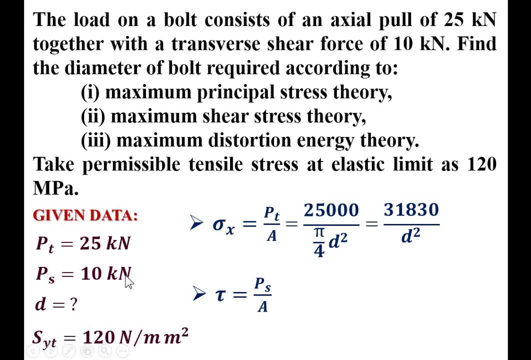 it is the shear stress, tau. so PS is given to you as 10 kilo Newton, so I can put it over here: 10 kilo Newton, that means 10. raise to 3 once again. shear area, that is pi by 4 D square for the. 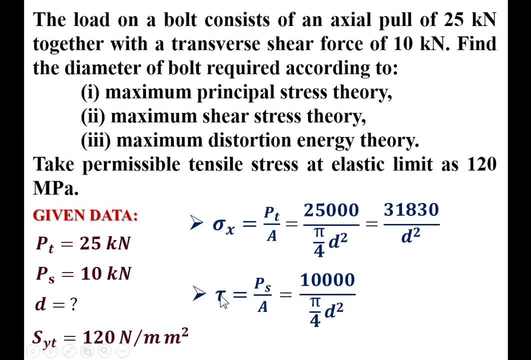 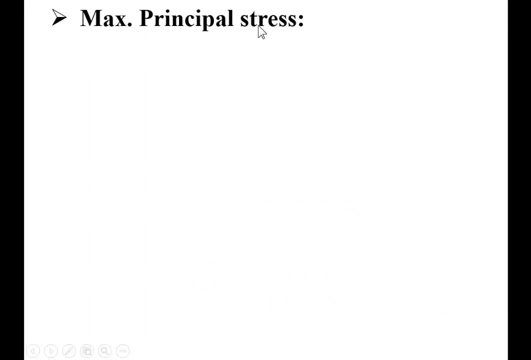 bolt. so if you simplify over here, then you will get tau in terms of D square. so once you got this- Sigma X and tau- that means the stress in x direction and shear stress- then I can find the maximum principal stress and minor principal stress. so let's start from. 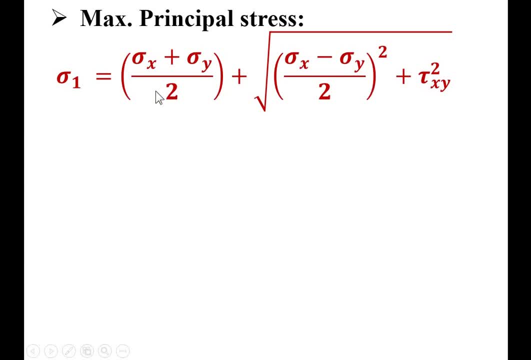 the first maximum principal stress. so, as we have discussed, this is the formula for the maximum principal stress. so here, Sigma Y is zero because of, in the description, the load that is not given to you in the y direction, and so that the stress in the y direction is zero. so, if you put it, Sigma, 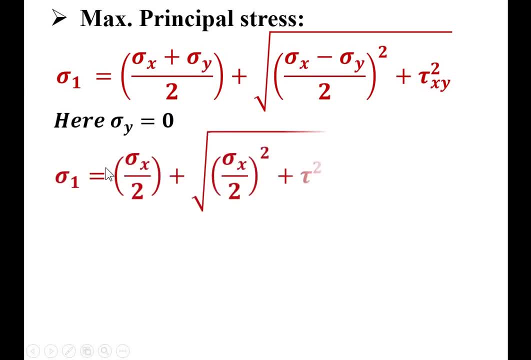 Y is equal to zero. so your Sigma one is only Sigma X by two plus square root of Sigma X by two, whole square plus tau square. so now I can put the value of Sigma X and tau in this equation. we have Sigma X and tau, so put this value both in. 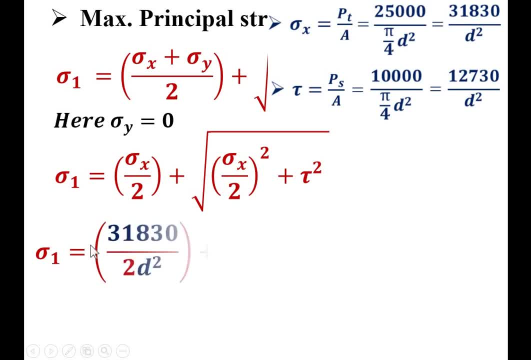 this equation so I can say Sigma one is, as it is, equal to Sigma X by two. so Sigma X is this one by two, as it is plus Sigma X by two, plus tau square. so I have used intentionally the different color. because of that, two is as it is. only we have put Sigma X with the blue color so you can understand easily. 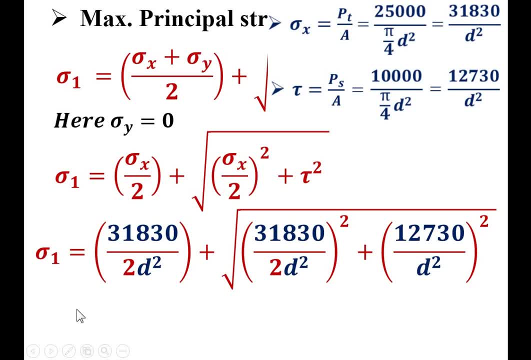 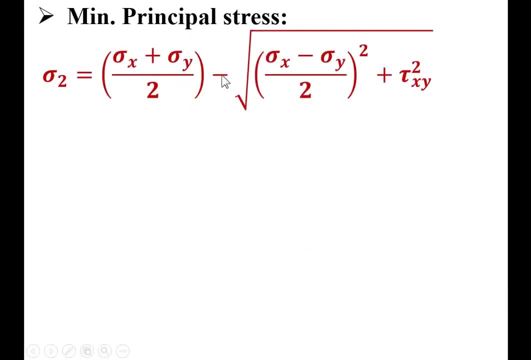 so if you simplify this whole equation, then you will get Sigma one in terms of diameter. so you will get this one. similarly, I can find minor principal stress now, but this again is for one factor. so the hum difference between the 2. you have Sigma x and 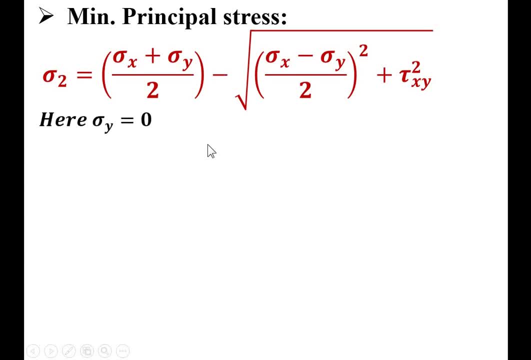 you will get this pin. so if you simplify the whole equation, you may predict the perception to be equal to two plus square root of sigma three. and let me share my deploying last part. basically, you can remember this function everywhere now. now when I am distributing all these values, I am, Например, of sigma 2. 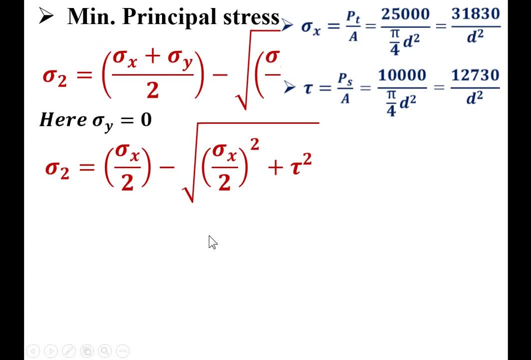 I can, Admitted it, that is what the sin against the Sachen here, that solution toız. so I have the give. I get this value give from sigma one, and then one любим that isanner principal stress at a Sigma two only, That is, sigma x and tau. 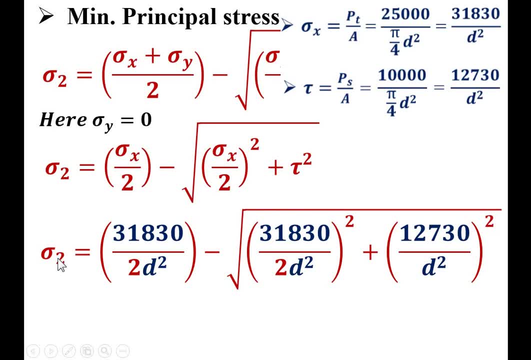 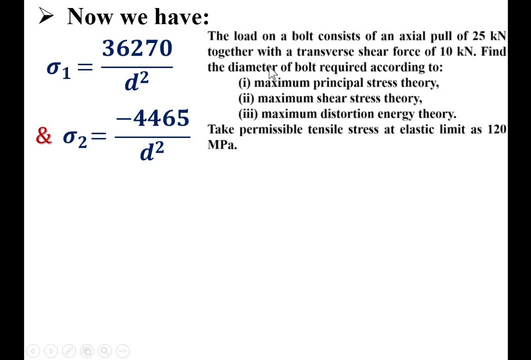 So if you simplify this equation, then you will get sigma2, that means minor principal stress in terms of diameter of the bolt. So here it is in negative value. So now look at this description. So now I can find the diameter of the bolt according to maximum principal stress theory. 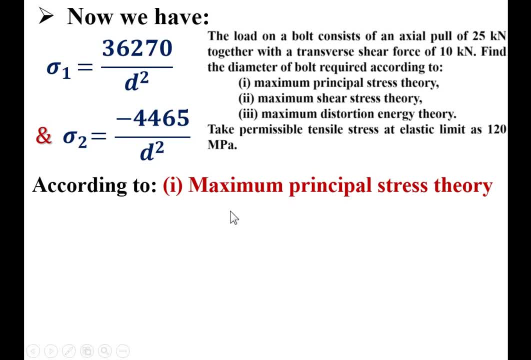 So according to maximum principal stress theory, as we have discussed in earlier videos of the theories of failure, that sigma1 is equal to Sy or Su upon NF. So that is the statement of the maximum principal stress theory. So here NF that means factor of safety. that is not given to you in your description. 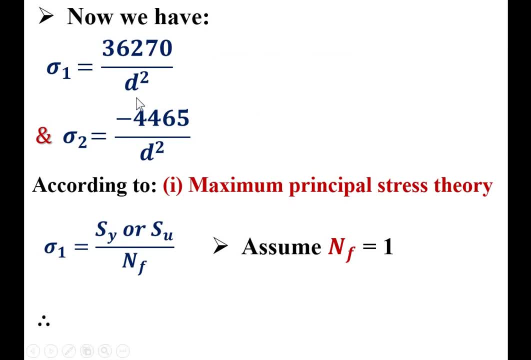 So you can assume as 1.. So sigma1 is this one, So I can put it over here- Is equal to Sy. that is also given to you in your description. That is sometimes known as Syt, So that is given to you in your description. 120, NF, we have assumed 1.. 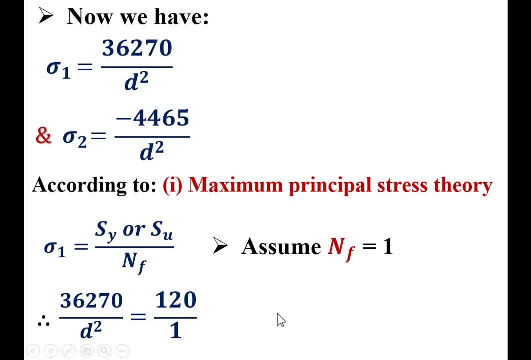 So if you simplify over here then you will get diameter of the bolt So it is 17.39.. So approximately you can say it is 18 mm. So that is your first answer. Diameter of bolt According to maximum Principal stress theory. 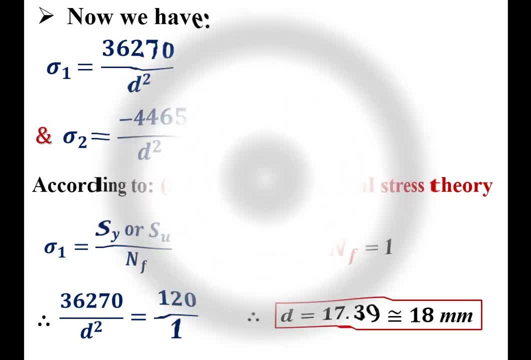 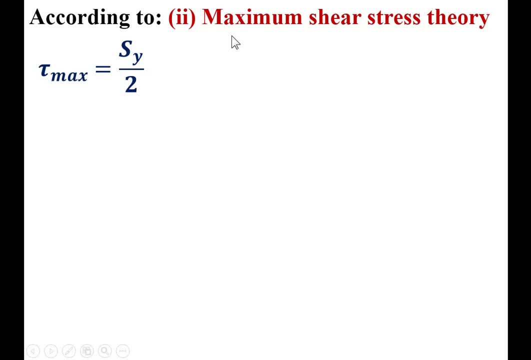 So make a box Now. next, according to maximum shear stress theory. So you know that the statement of the maximum shear stress theory that tau max is exactly equal to Sy by 2.. But for that you have to find the tau max And as we have discussed that maximum shear stress, tau max is equal to sigma1 minus sigma2. 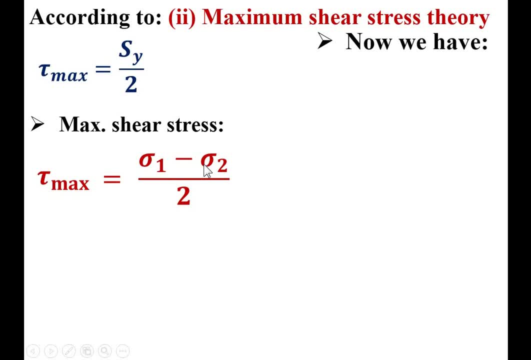 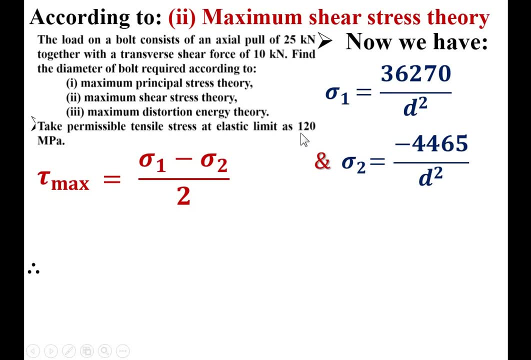 by 2. And already you have sigma1 and sigma2.. And maximum shear stress is directly not given to in your description But it is given to as tensile stress And majority of the metal. maximum shear stress is half of the tensile stress. 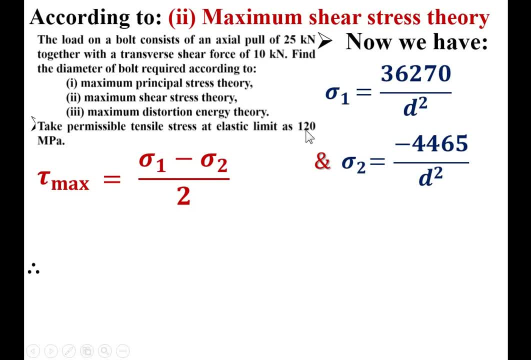 So I can say: tau max is half of this tensile stress, So it is 120 by 2 is equal to sigma1. That is this one Minus F1.. Minus F2.. And size: it is sigma2.. That is this one divided by 2.. 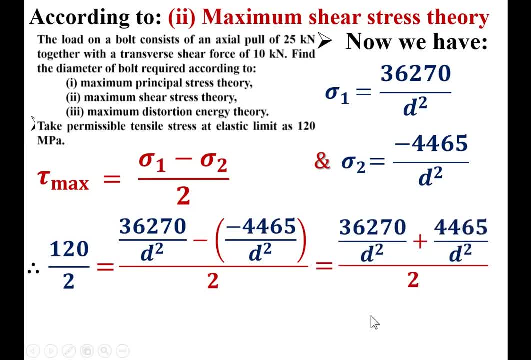 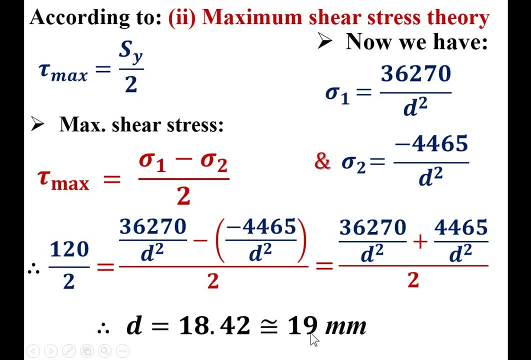 So this is minus minus plus, And so that you will get the diameter, And that is 18.42.. And so that nearly equal to you can say 19 mm. So this is your second answer, according to maximum shear stress theory. So make a box. 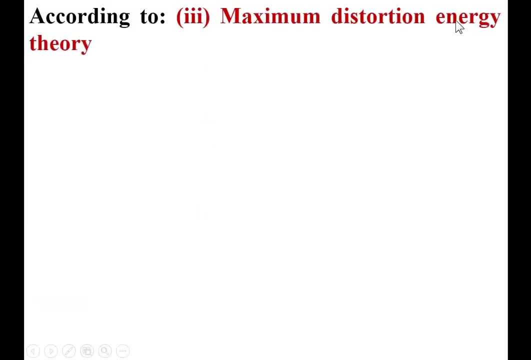 Now third one, According to maximum Distortion energy theory. So this is the statement of the maximum distortion energy theory. So we have sigma1.. We have sigma2.. We have SyT, also 120.. So now I can put it over here in this equation: 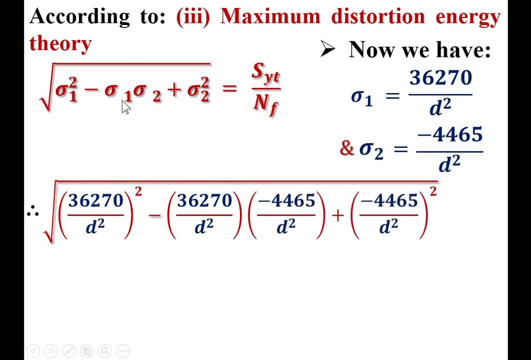 So sigma1 whole square, That means this one whole square, Minus, as it is, sigma1 into sigma2.. So this is sigma1 and sigma2.. Plus Sigma2 whole square That is equal to SyT That is given to in your description as 120.. 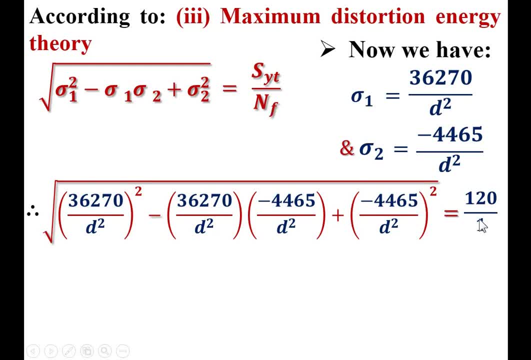 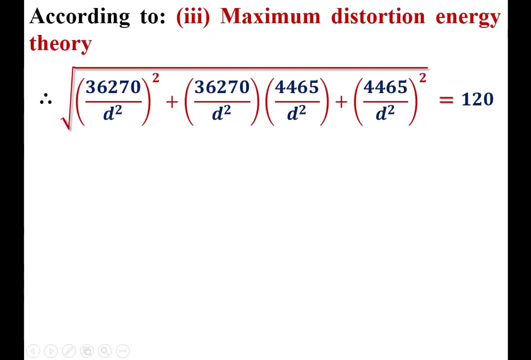 Divided by NF, Factor of safety. That is not given to you, So you can assume as 1.. But once again, keep in mind that minus, minus will be plus over here And that is exactly equal to 120.. So already we have discussed up to here in the earlier slide. 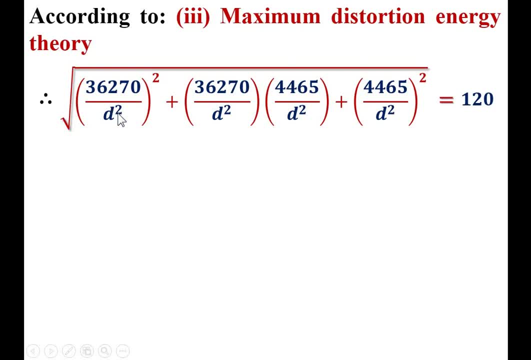 Now, if you simplify on this side, then you will get this: one is equal to 120, as it is. So if you simplify this equation, then you will get diameter of the bolt, and that is 18.43, and that is nearly equal to 19 mm. 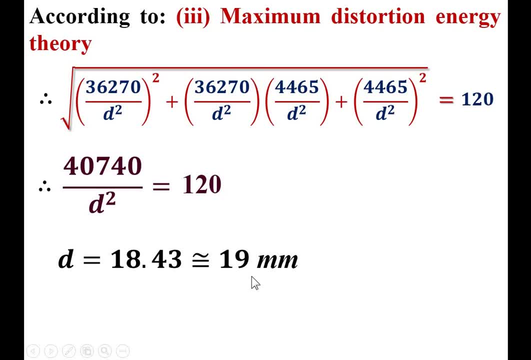 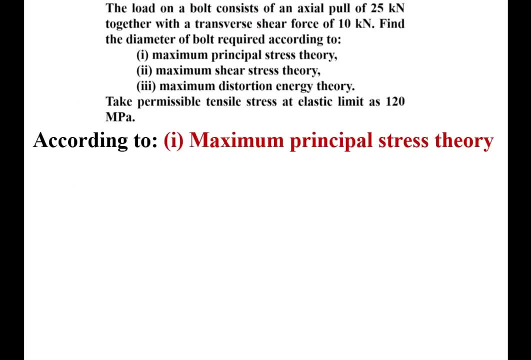 So this is your third answer. according to maximum distortion energy theory. So make a box. So now You can summarize over here. This is your description And these are the objective. So first one: according to maximum principle stress theory, this is the diameter. 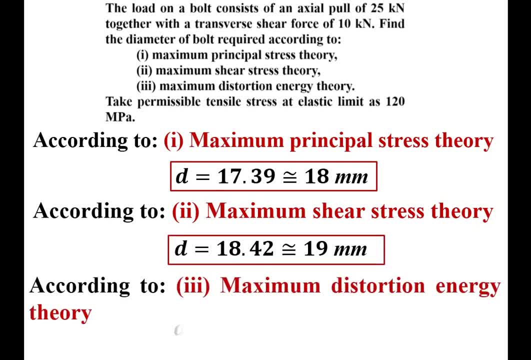 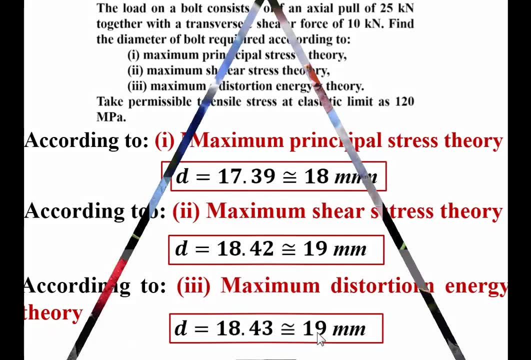 According to maximum shear stress theory, this is the diameter. And according to maximum distortion energy theory, this is the diameter. So thanks, my dear friends. Press the like button to appreciate this video. 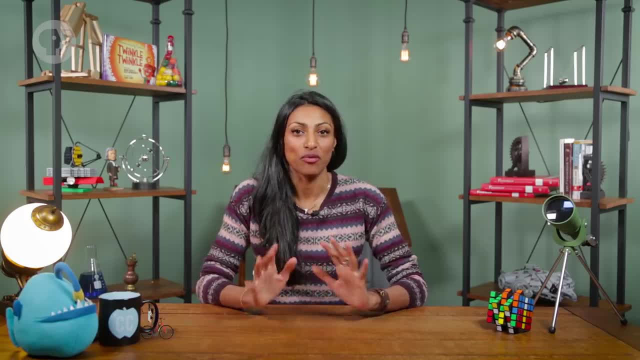 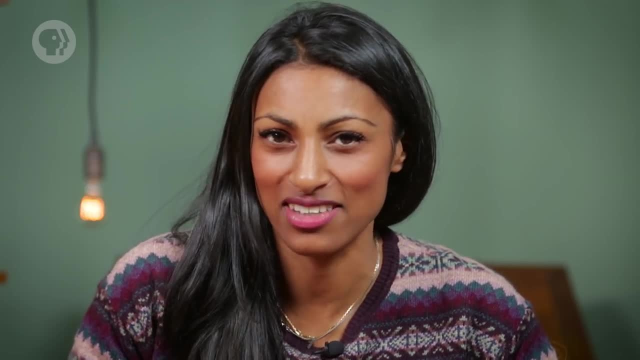 So far, we've spent a lot of time predicting movement – where things are, where they're going and how quickly they're going to get there. But there's something missing, and something that has a lot to do with Harry Styles And 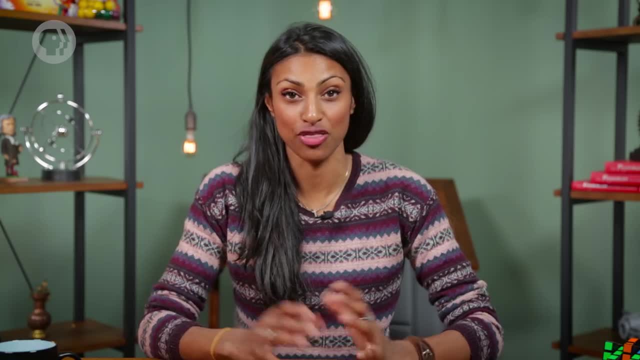 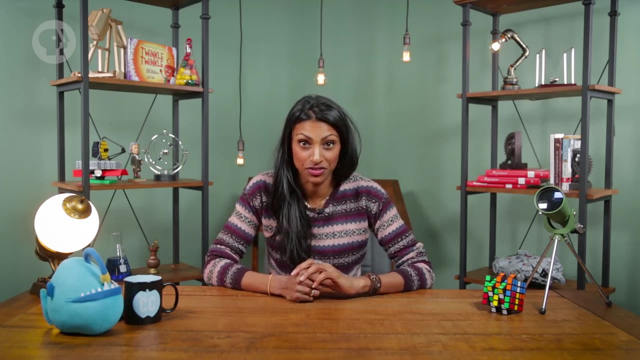 today we're going to address that. We've been talking about what happens when you do things like throw balls up in the air or drive a car down a straight road. That kind of motion is pretty simple because there's only one axis involved: The car's. accelerating either forward or backward. the ball's moving up or down. there's no messy second dimension to contend with. But this is physics. We may simplify calculations a lot of the time, but we still want to describe the real world as best we can. 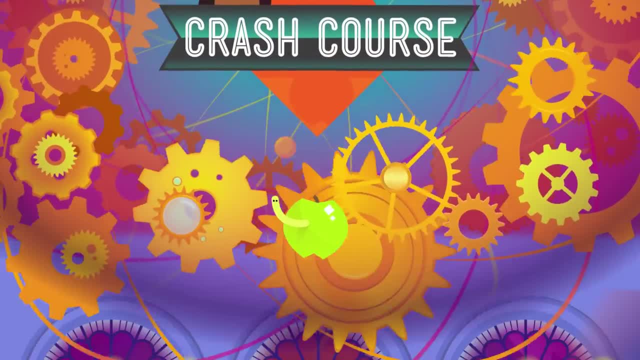 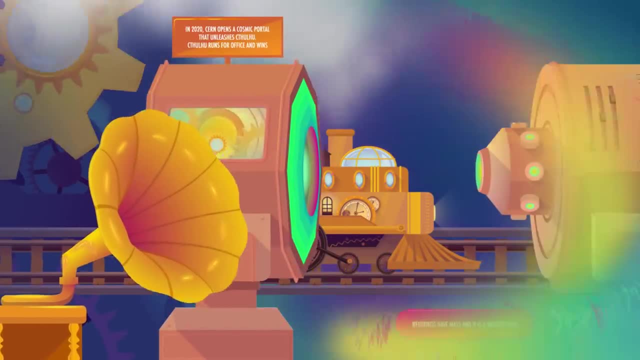 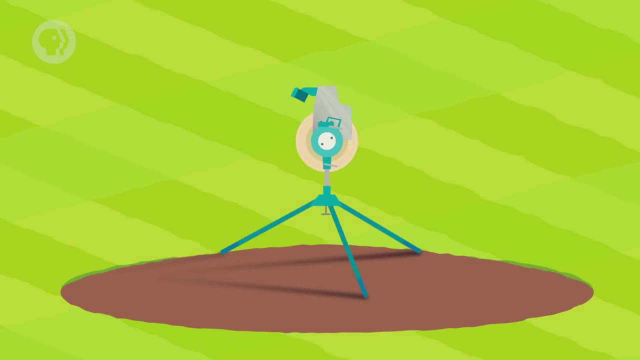 And in real life, when you need more than one direction, you turn to vectors. Let's say, we have a pitching machine like you'd use for baseball practice. We're going to use it a lot in this episode, so we might as well get familiar with how it works. 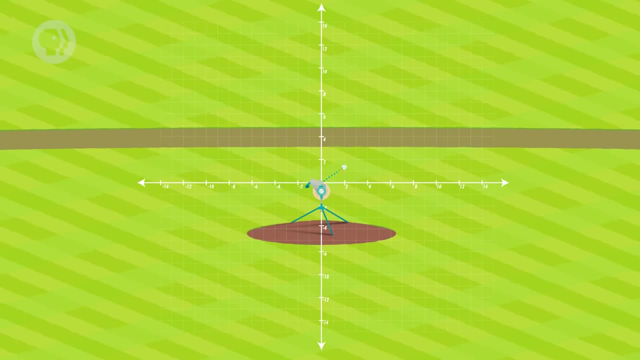 We can feed the machine a bunch of baseball balls and have it spit them out at any speed we want, up to 50 meters per second. The pitching height is adjustable and we can rotate it vertically so the ball can be launched at any angle. 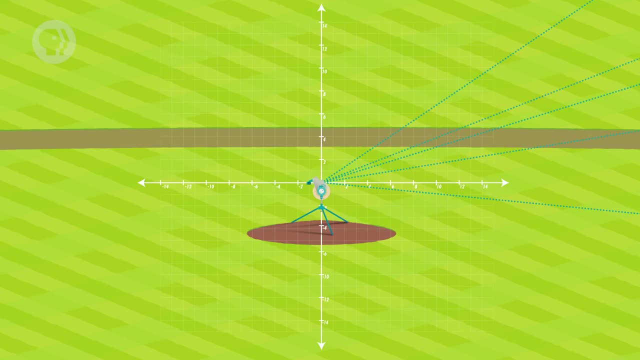 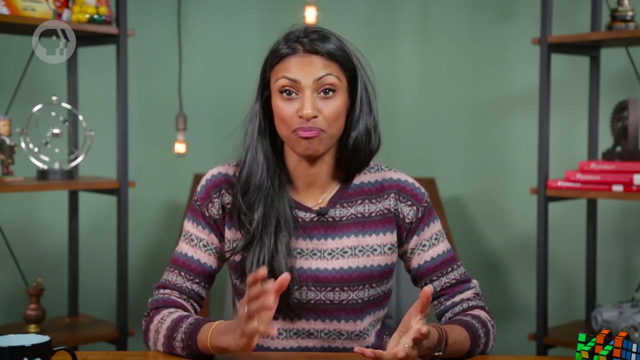 It also has a random setting where the machine picks the speed, height or angle of the ball all on its own. Suddenly, we have way more options than just throwing a ball straight up in the air, And now the ball can have both horizontal and vertical qualities at the same time.